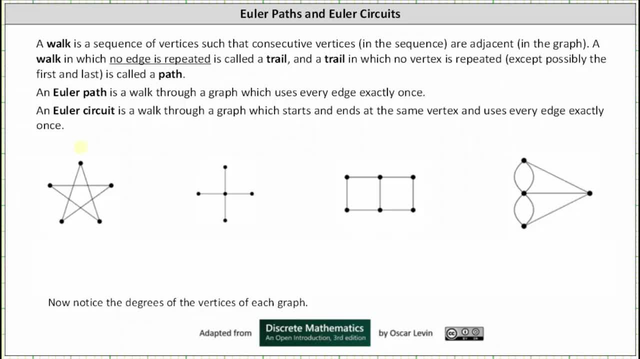 and start at this top vertex. We'll label it S to indicate where we're starting. And now we determine if there's a walk through the graph which uses every edge exactly once, And we typically use arrows or numbers to show the direction of the walk. I'm going to go ahead and 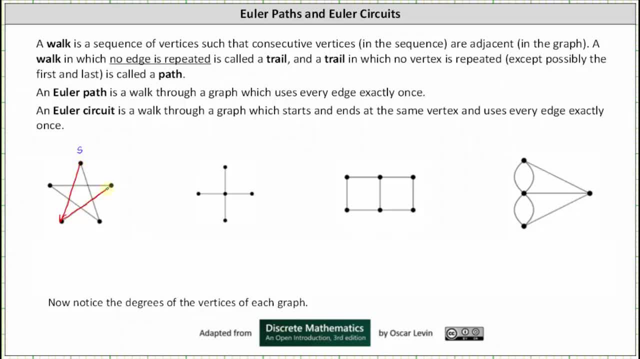 use arrows, Because each vertex has degree two. once we start, there's no question in which direction to walk. Notice the walk is now complete and we used every edge and every edge exactly once. This indicates the graph has an Euler path. We also started and ended at the. 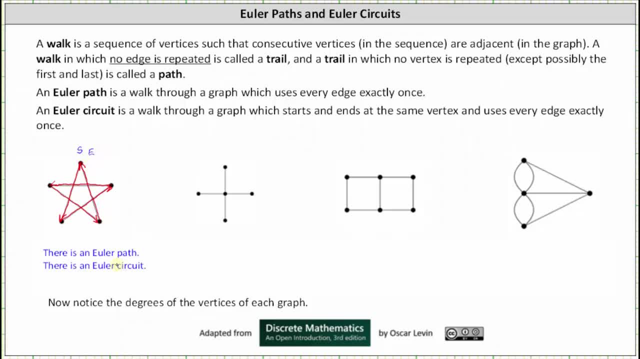 same vertex. The graph also has an Euler circuit. Looking at the next graph, let's start the walk at the top vertex And now we walk through the graph and see if we can use every edge exactly once So we can go down. We need to decide whether to go left, right or down In this case. 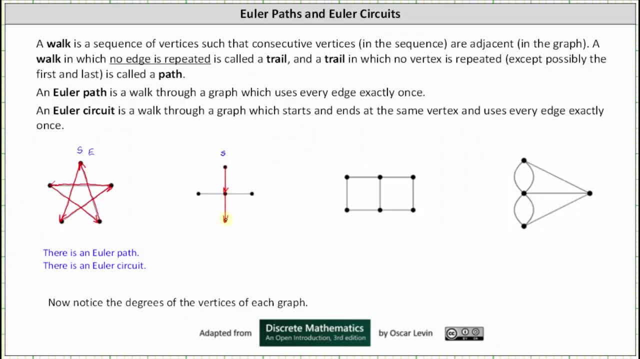 it doesn't matter Whichever direction we go, we get stuck. We cannot continue the walk unless we repeat an edge, which is not allowed. This doesn't mean the graph doesn't have an Euler path or circuit. We can try starting from a different vertex. 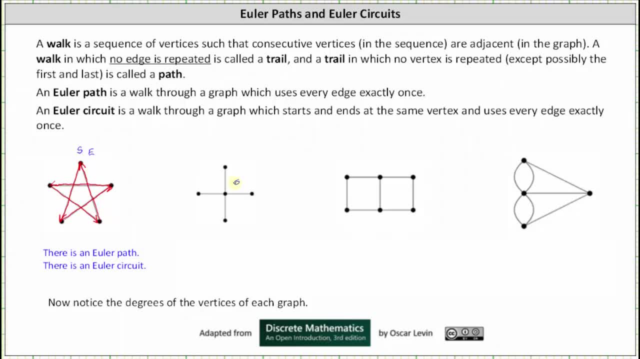 So let's try starting at the vertex in the middle. But we do run into the same problem: Whichever direction we go, we get stuck. The walk cannot continue unless we repeat an edge, which again is not allowed. The graph has no Euler path and no Euler circuit. 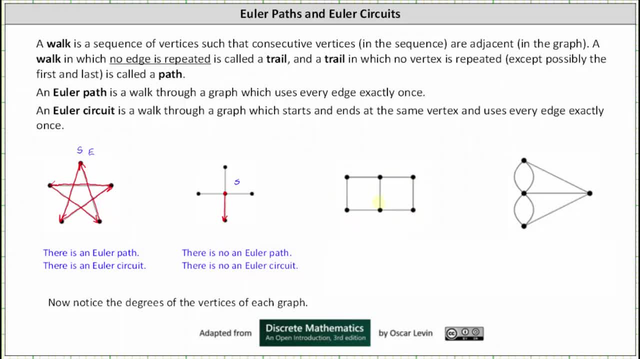 Looking at the next graph, notice how four the vertices have degree two and two of them have degree three. Let's try starting at a vertex with an even degree. let's say, here And now we walk through the graph. Let's go right, right down, left. 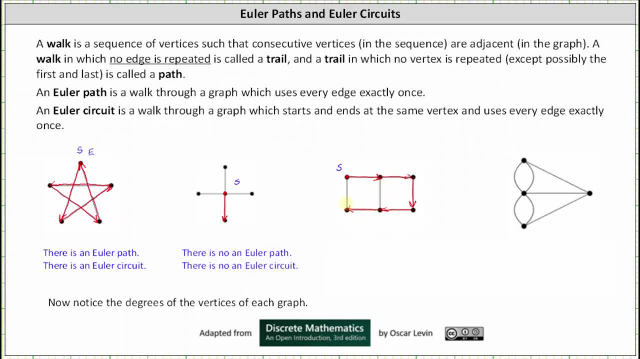 If we go up we're going to get stuck, so let's go left again. Then we have to go up and we're stuck again. The walk cannot continue unless we repeat an edge, which again is not allowed Again. that doesn't mean the graph doesn't have. 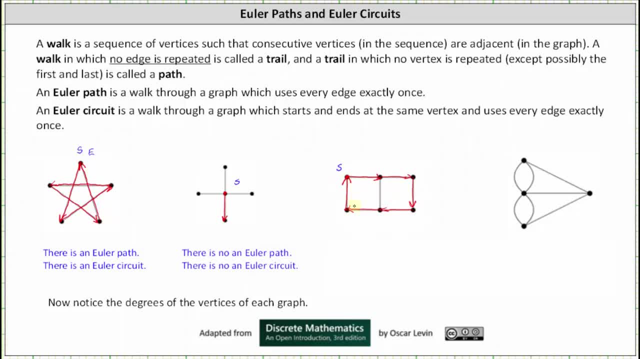 an Euler path or Euler circuit. We can try starting from a different vertex. So let's try starting with one of the vertices that have an odd degree, Let's say this middle vertex. here Let's start the walk. Let's go right down left. 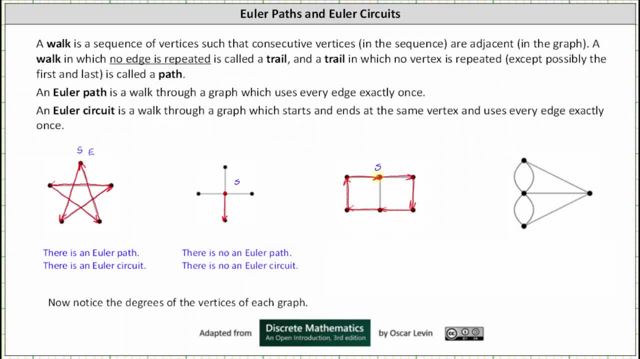 left up, right down, And now we end the walk. We were able to walk through the graph using every edge, exactly once The graph has an Euler path. However, we did not start and end at the same vertex. The graph does not have an Euler circuit. 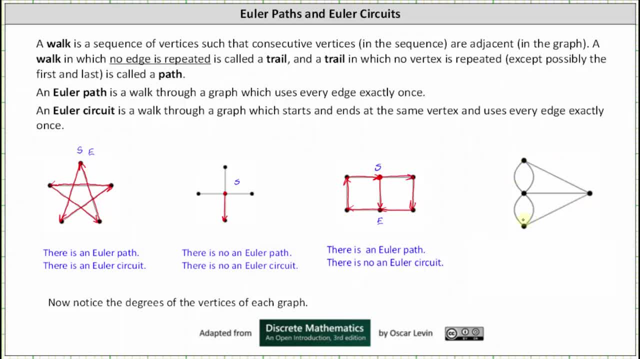 For the last graph. we should recognize this as the graph from the seven bridges of Konigsberg problem. Let's try starting at this top vertex. And now we walk through the graph and go down Down. let's go up up, right. 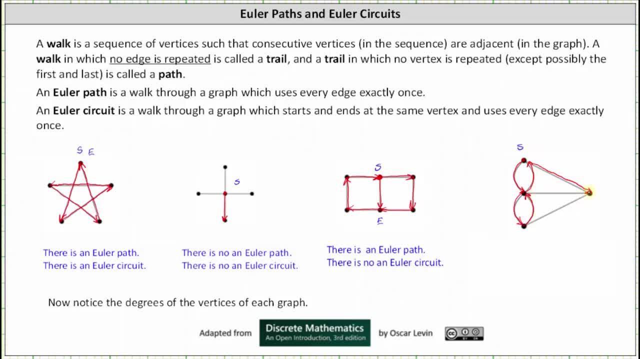 Now, when you decide whether to go left or down, either way we're going to get stuck again. If we go left, the walk cannot continue unless we repeat an edge, which again is not allowed. The same thing would happen if we went down instead of left. 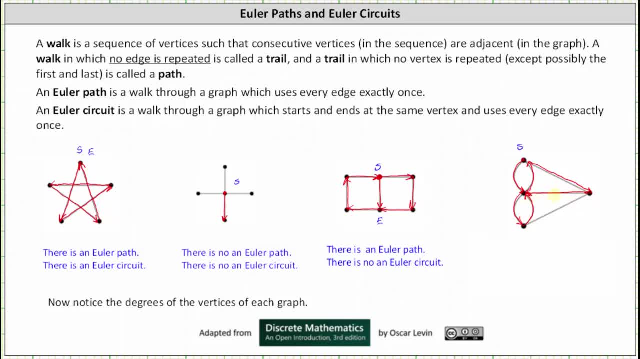 So you may want to try this a few more times, but this graph does not have an Euler path. It also doesn't have an Euler circuit. Before we go on, let's check the degrees of all the vertices and see if we can find any differences. 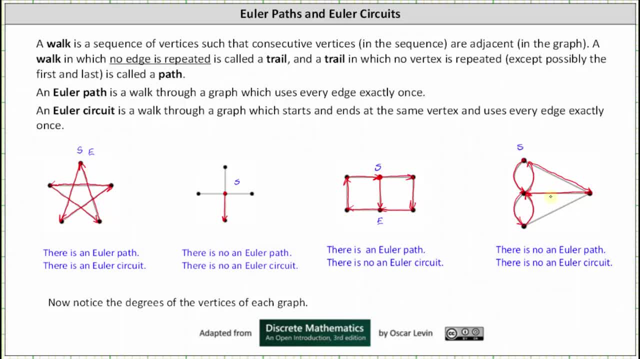 But before we go on, let's check the degrees of all the vertices, vertices and the graphs. There is a connection between the degrees of the vertices and whether a graph has another path and or another circuit. Going back to the graph on the left, all the 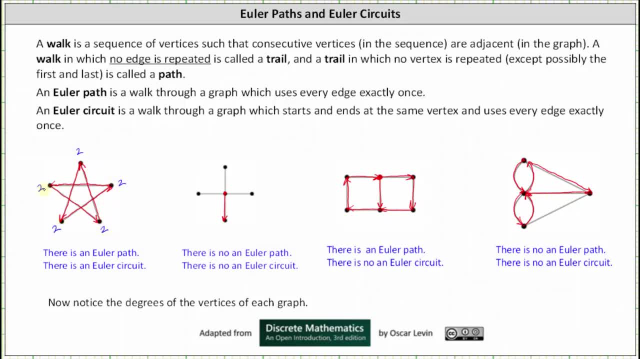 vertices have degree two, or we can say all the vertices had an even degree and the graph had both another path and another circuit. For the next graph, four of the vertices have degree one and one of them has degree four. We have four vertices with an odd degree, one with an even. 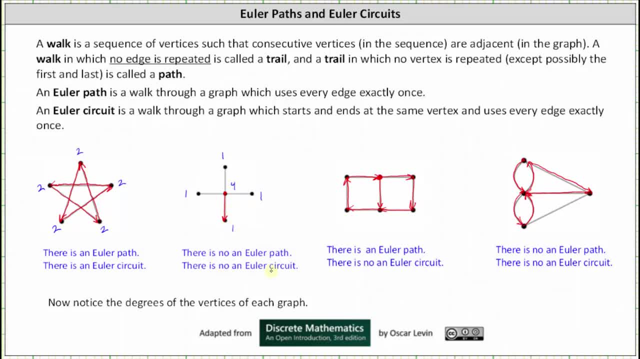 degree and the graph had no other path and no other circuit. For the next graph, four of the vertices have degree two and two of them have degree three. We can say four of the vertices have an even degree, two of them have an odd degree and the graph had no other path but no. 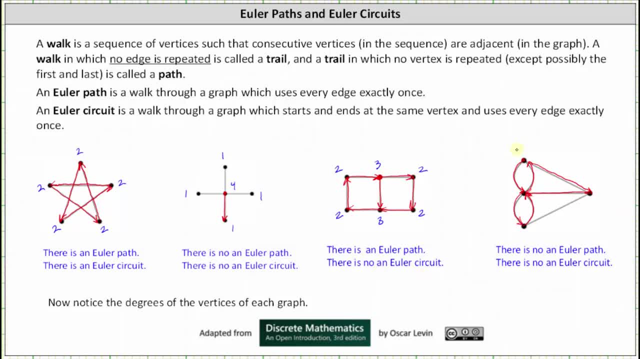 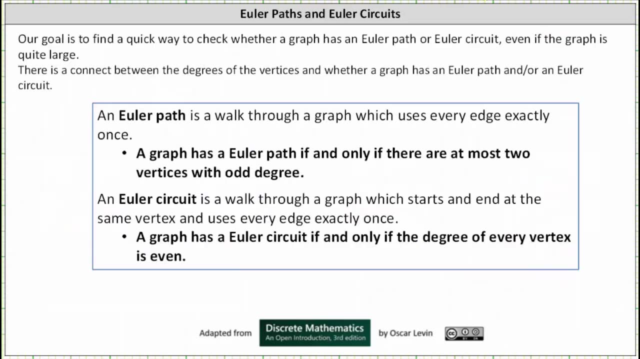 other circuit And for the last graph the degrees are three, three, three and five. All the vertices have odd degrees and the graph had no other path and no other circuit. So again, the goal here is to find a quick way to check whether a graph has. 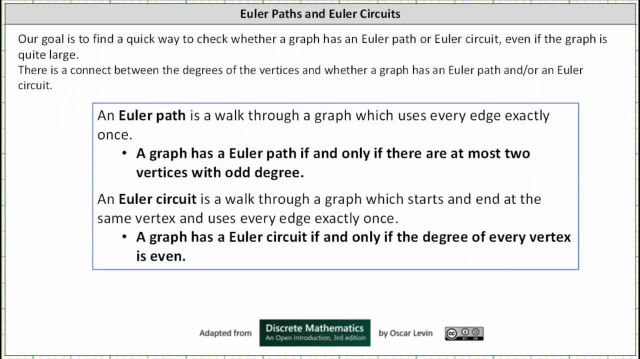 another path or another circuit, even if the graph is quite large. And again, there is a connection between the degrees of the vertices and whether a graph has another path and or another circuit. A graph has another path if, and only if, there are most degrees of the vertices. And to golfer the graph, we click on the lower left corner of the. 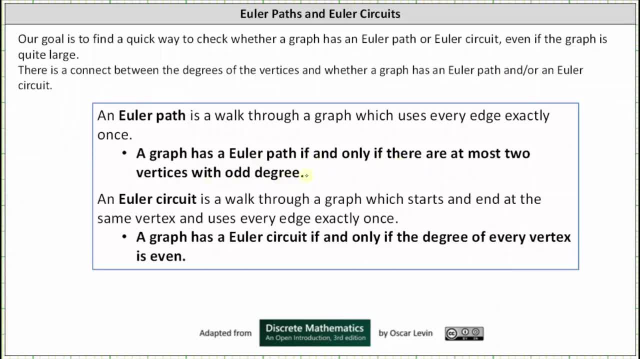 graph: If, and only if, there are mountains of vertically 39,ue Connected Vertices, If, and only if most two vertices with odd degree. So if all the vertices have an even degree, or at most two vertices have an odd degree, then the graph will have an Euler path. 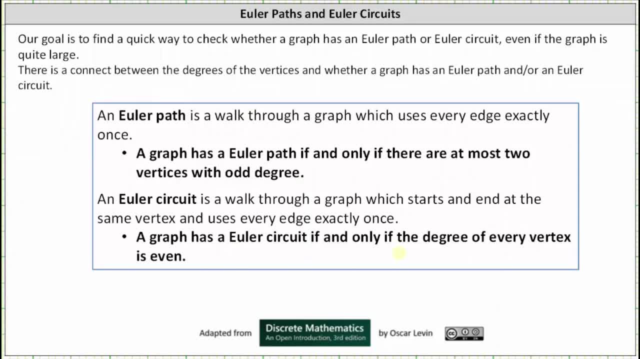 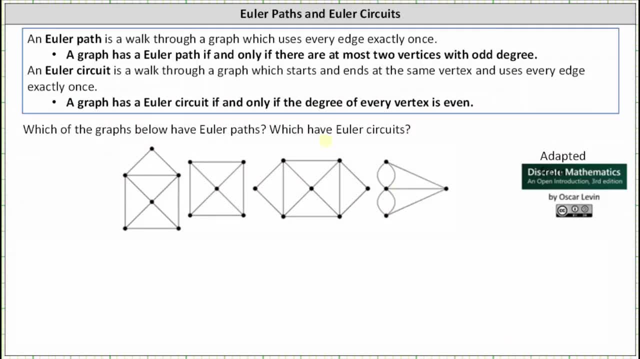 A graph has an Euler circuit if, and only if, the degree of every vertex is even. Let's take a look at four more graphs and determine whether they have Euler paths and or other circuits now, by analyzing the degrees of the vertices, Starting with the graph on the left. 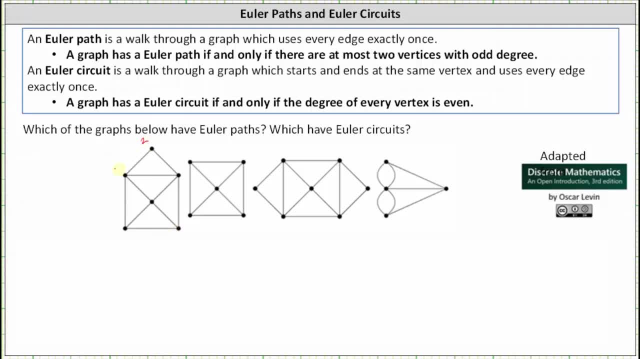 let's find all the degrees of the vertices. We have degree two, degree four, degree three, degree three, degree four and degree four. The graph has four vertices with even degree and two vertices with odd degree, Because the graph does satisfy the condition. 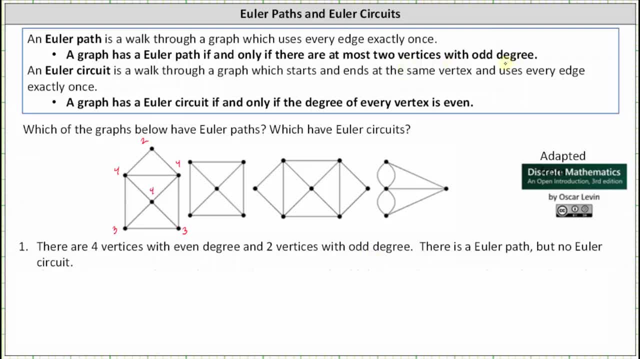 of having at most two vertices with odd degree. the graph has an Euler path but no other circuit, because all the degrees are not even Looking at the next graph, we have degree three, degree three, degree four, degree three and degree three. 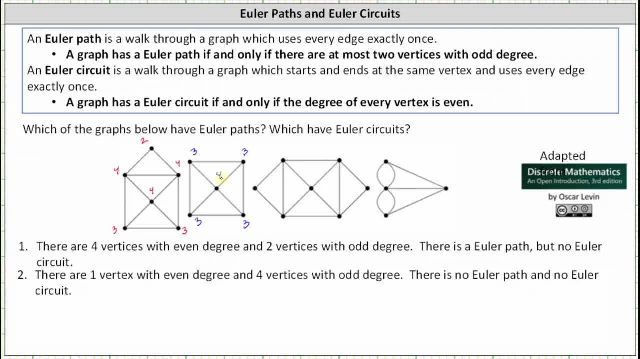 One vertex has an even degree, Four vertices. four vertices have an odd degree. because more than two vertices have an odd degree, the graph does not have an Euler path and also does not have an Euler circuit. Whenever a graph doesn't have an Euler path, 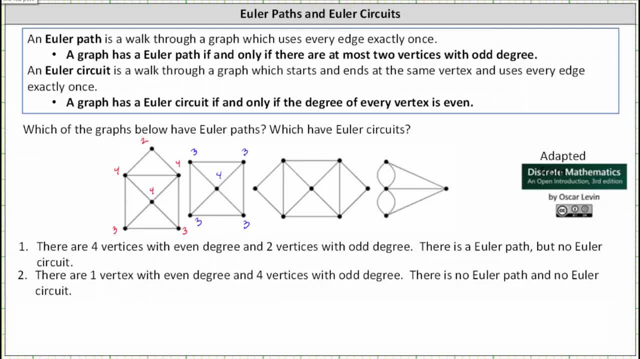 it will never have an Euler circuit. And for the next graph we have degree two, degree four, degree four, degree two, degree four, degree four and degree four. All seven vertices have an even degree. This indicates the graph has both an Euler path. 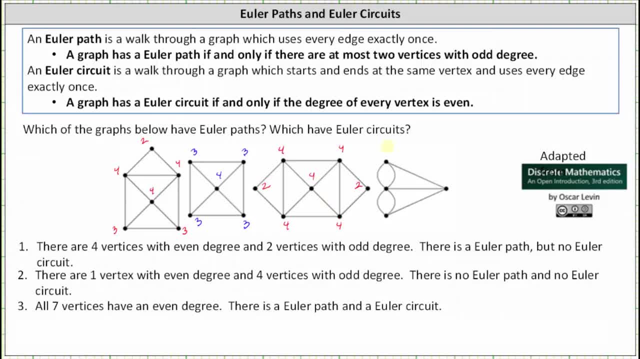 and an Euler circuit. And then for the final graph, we have degree three, degree three, degree three and degree five. All four vertices have an odd degree. We have more than two vertices with an odd degree. The graph does not have an Euler path. 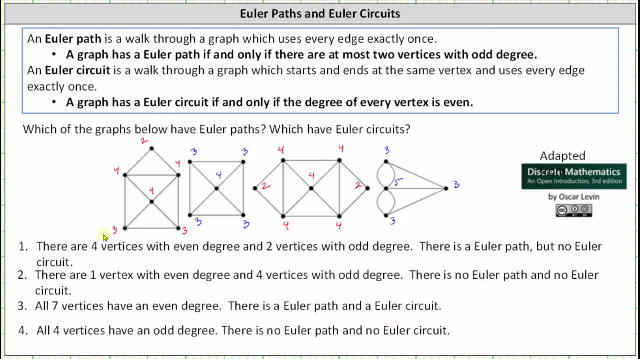 and also does not have an Euler circuit. I hope you found this helpful.